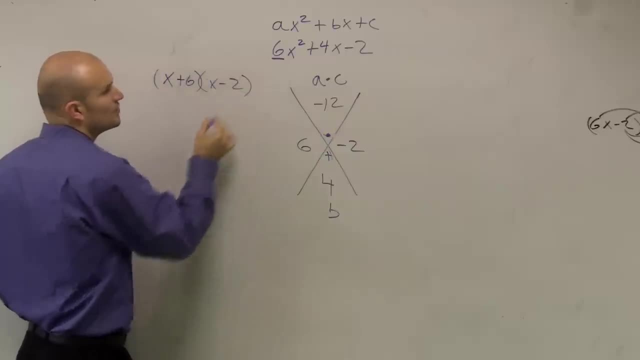 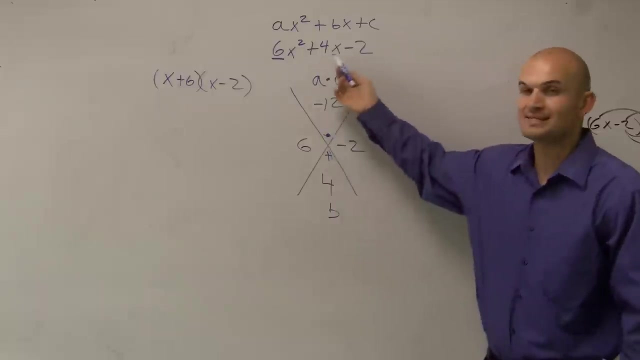 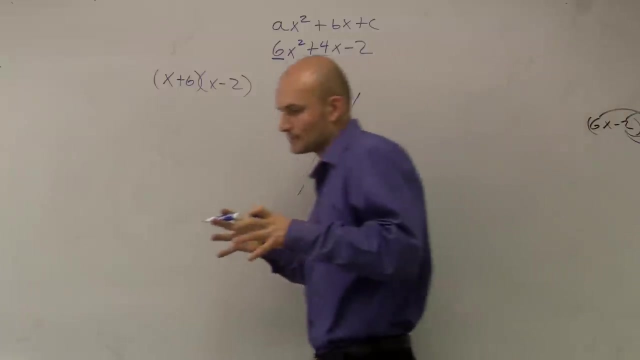 it's going to be x plus 6 times x minus 2, because that is not the same. Remember as a product, remember as a well. when I say factory, we're writing this as a product of its two factors. The mathematical equivalent has not changed The mathematical I'm losing. 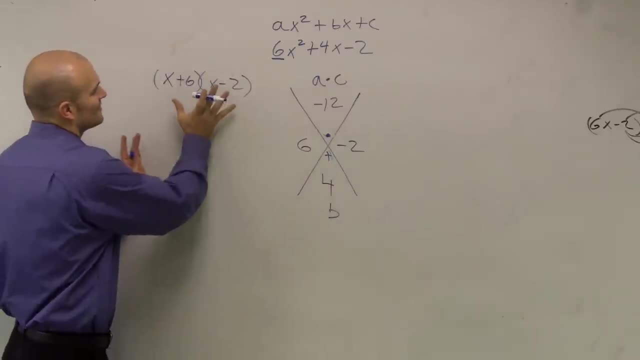 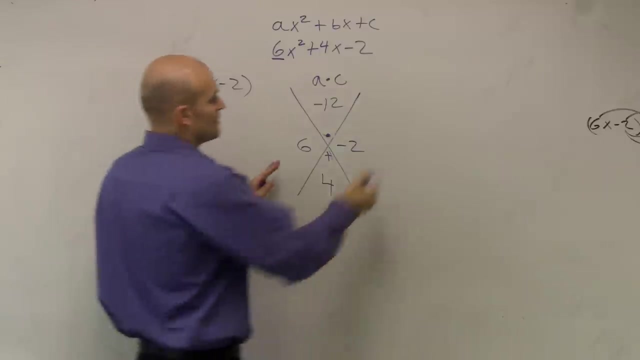 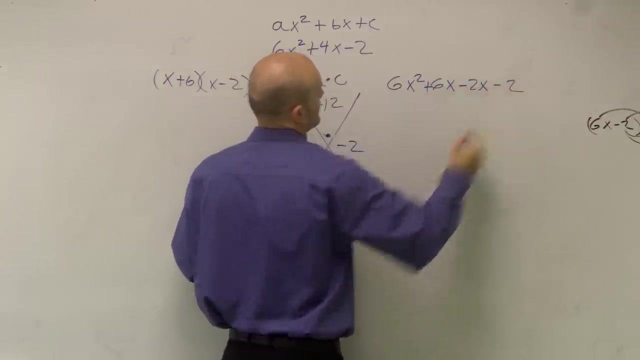 my train of thought. but the value of the mathematical expression does not change. This does not multiply to give me that. So what I'm going to do is I'm just going to rewrite my middle terms. So when I rewrite my middle terms now, this has the same value. 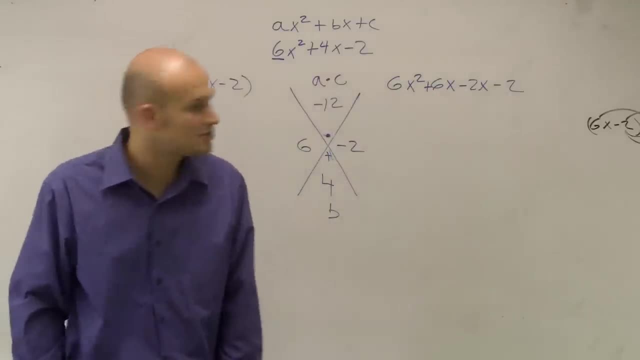 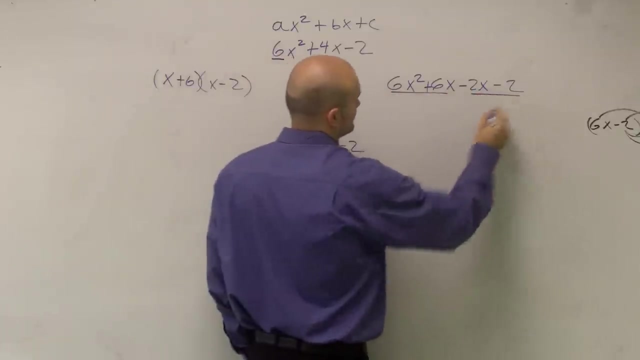 All I did was replace a 4x with a 6x minus 2x minus 2.. Now what I can do is I can factor each one of these terms. All right, so I'm going to factor the first two terms and the. 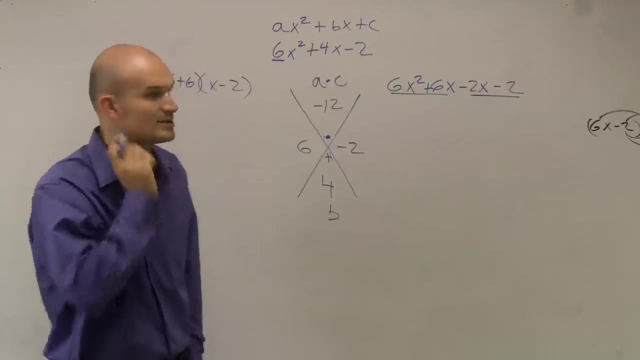 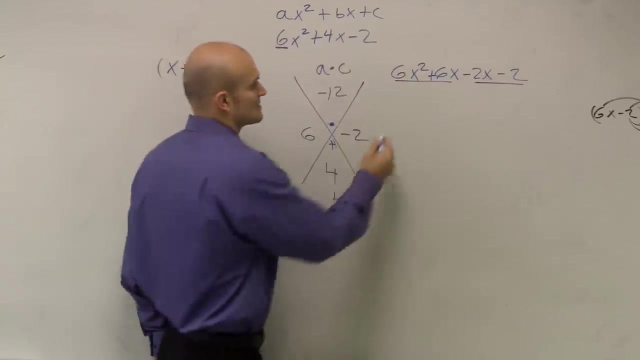 last two terms. When I factor the first two terms, I look at what is a 6x squared plus a 6x. What do those have in common? Well, these two terms, they both have in common a 6 and an x. So when I factor out a 6x, the first thing I'm thinking of is: you know. 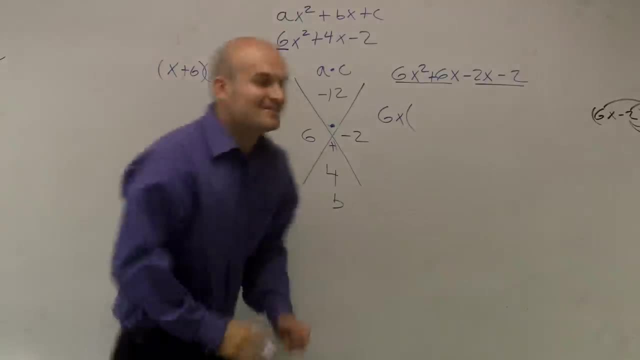 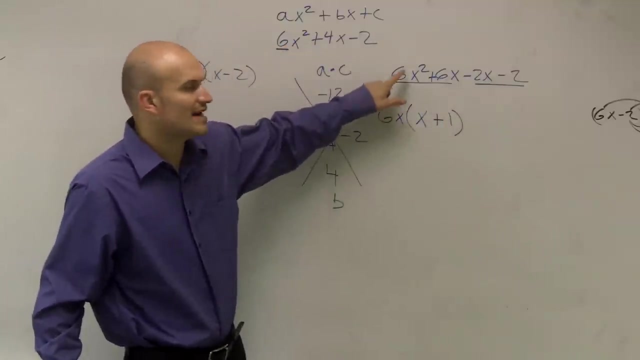 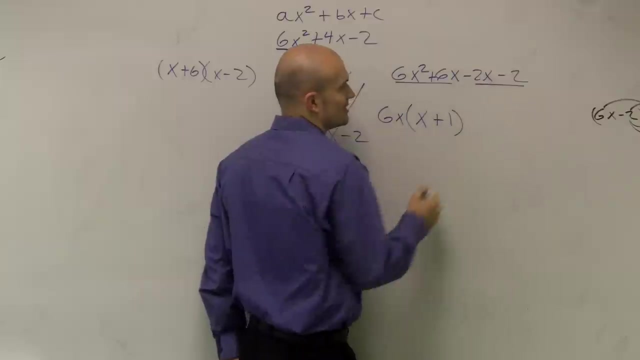 when I divide out a 6x, what I'm left with is an x plus 1.. All right, because 6x evenly divides into 6x squared plus 6x When it divides into it, my result is an x plus 1.. Here I 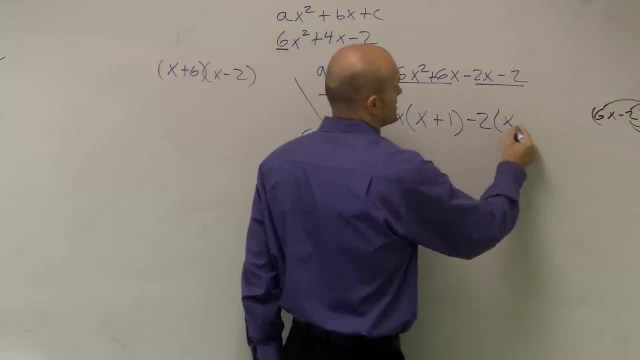 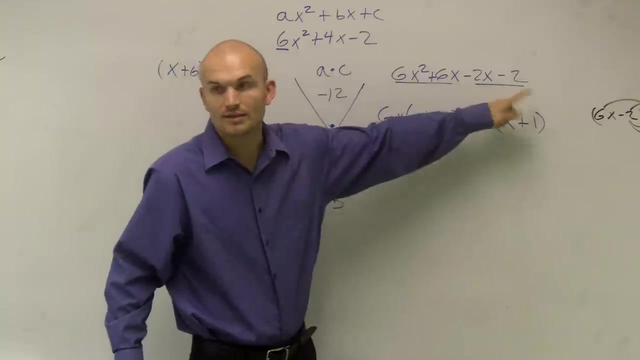 can now divide out a negative 2 times x plus 1.. So it's important from this point on. so, since I divide out a negative 2, because that's the only thing that these two the terms have in common- is a negative 2. When I factor out my negative 2, now I'm left with 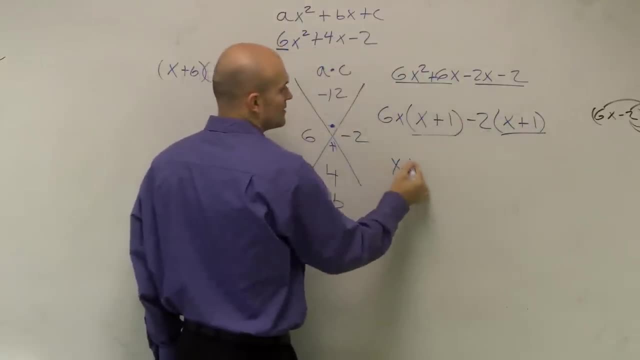 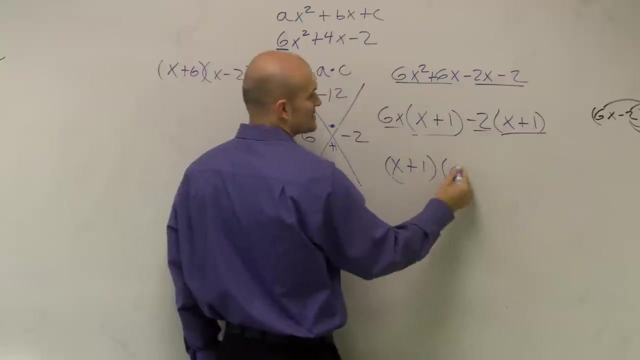 an x plus 1 and an x plus 1.. I can now factor those out to give me x plus 1 times. after I factor these two out, I'm left with a 6x minus 2. And that is how you factor when you. have an a greater than 1..